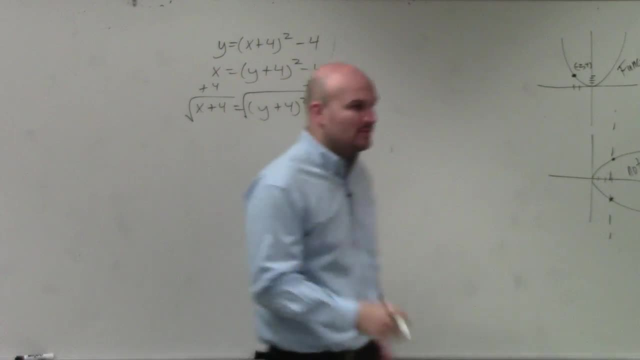 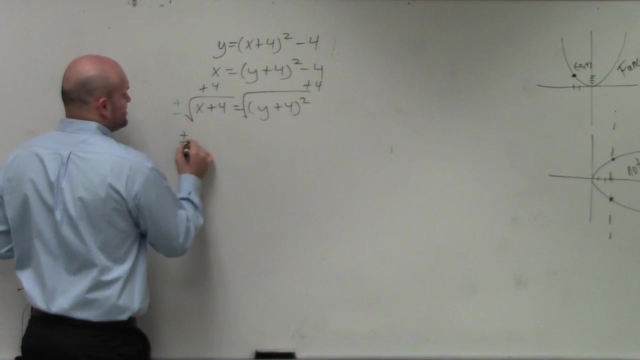 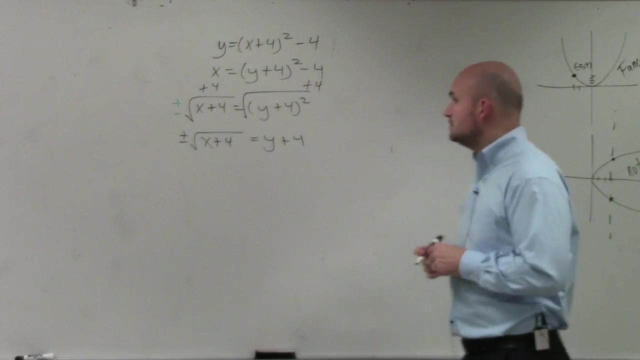 the parentheses. so I take the square root of both sides. Please remember, when you introduce the square root you have to do the plus or minus. So I have, plus or minus, the square root of x plus 4 equals y plus 4.. How do I distribute what? 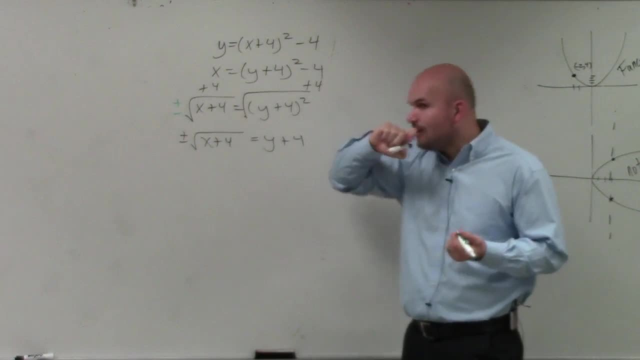 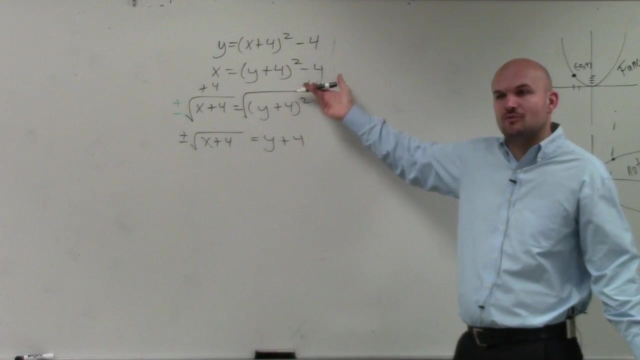 You could. You could, but you're trying to solve for y. So distributing is going to make that y squared plus 4y plus 16.. It's not really going to help you solve for y. To solve for y you're trying to. 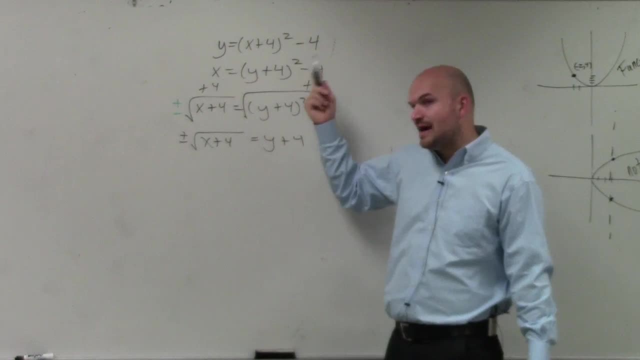 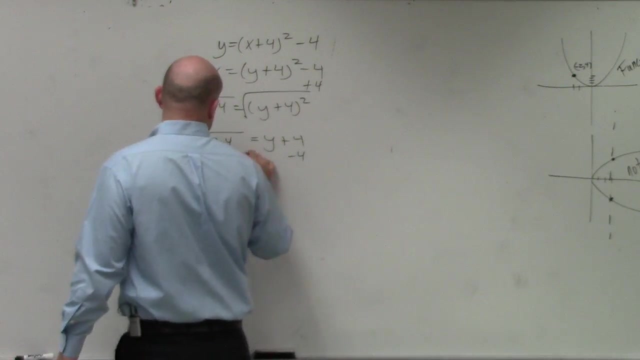 undo everything that's happening to it, right? So rather than applying squaring, I want to undo the squaring by taking the square root. Does that kind of make sense? So now I just subtract the 4, and I have plus or minus the square root of x squared. 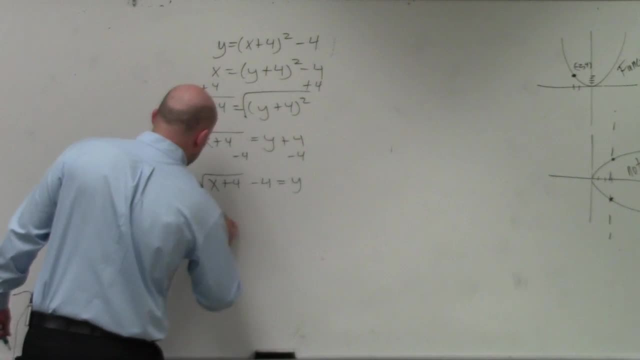 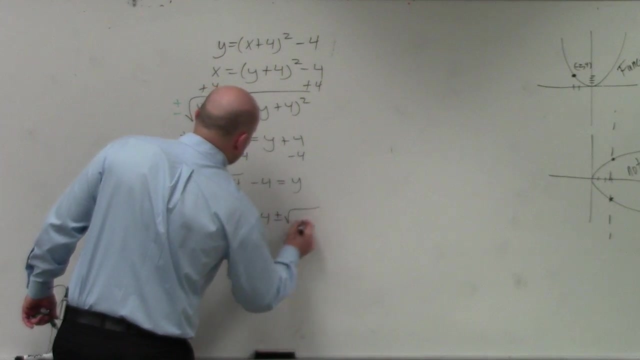 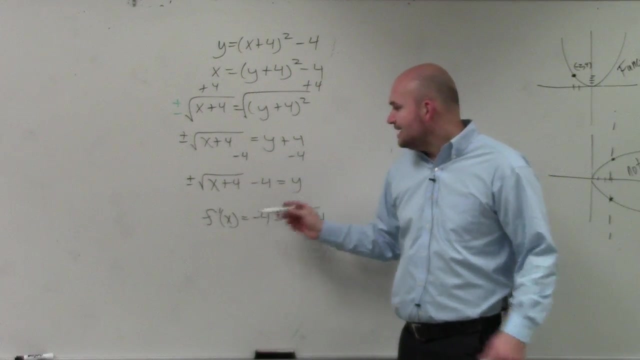 So now I have plus or minus the square root of x plus 4 minus 4 equals y. or I could write: f inverse of x is equal to negative, 4 plus or minus the square root of x plus 4.. So therefore, now what I basically did is I just rewrote my y as f inverse of x equals negative 4 plus or minus the square root of x plus 4.. 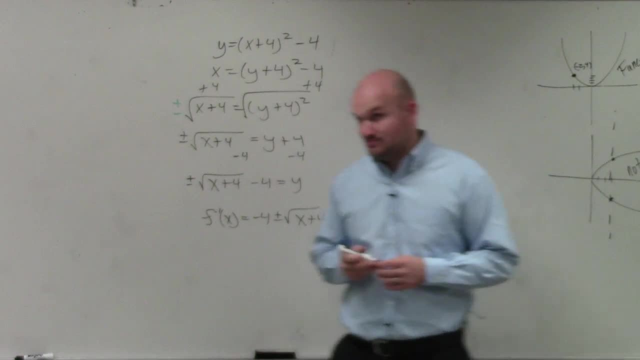 Now, if you guys look at this problem, if I choose a number for x, right, Let's choose the number 0 again. If you plug in 0 into this function, are you going to have? is there a problem? If you plug in 0 into this function, are you going to have? is there a problem? 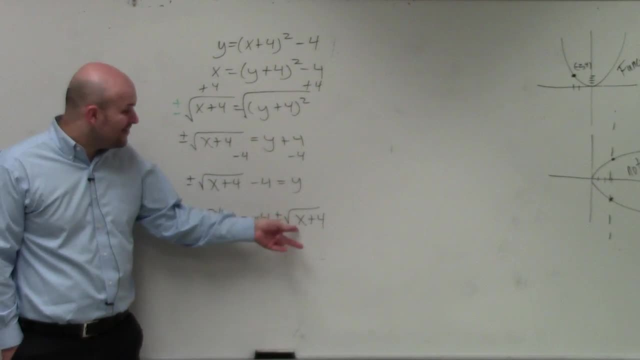 Yes, because now you have to do plus or minus. You guys see that. So anytime you are solving for the function and you include a plus or minus, that is not going to give you your function or, sorry, your inverse is not a function. 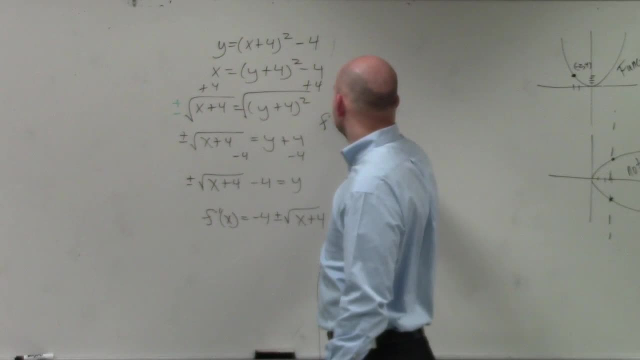 So you could just basically write f inverse is not a function, or answer for b section it would be no. Do you guys kind of see the difference between those two? The first example: whatever you plugged in for x, you're going to get an answer for y. That's a function.